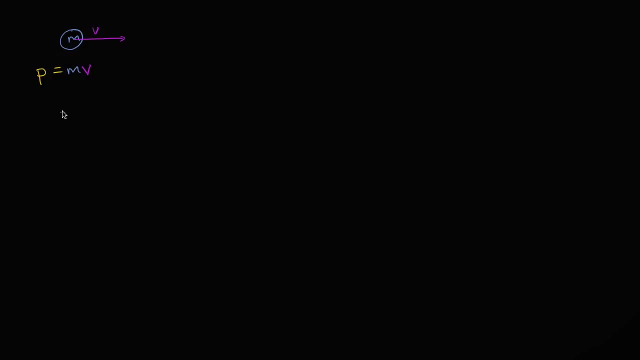 I mean you literally, in everyday language. you think, well, how much momentum does something have? The more momentum it has, the harder it's going to, the harder it is to stop it in some way. And so we know if we wanna get a little bit. 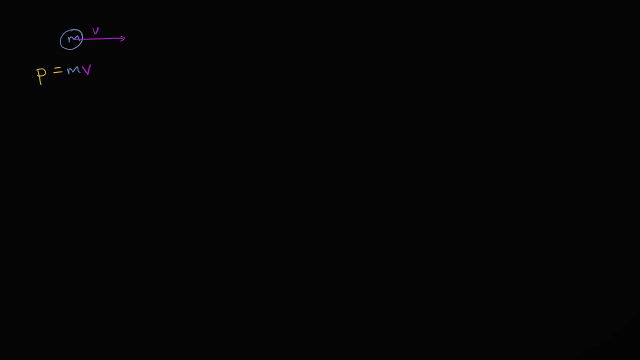 more mathematical that if we wanna change momentum, we have to apply force for some amount of time, And so the magnitude of our force, the magnitude of our force, times the duration of the time that we apply it, for force times time, and this is called impulse. 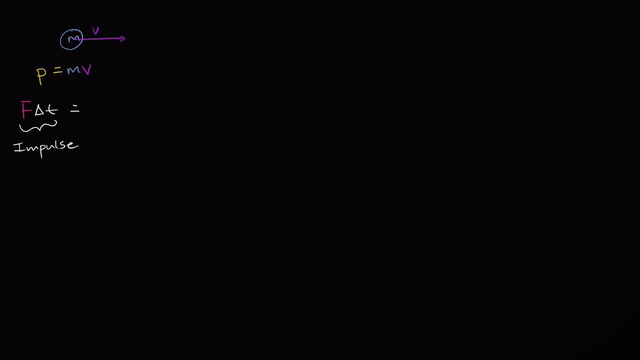 And this is once again all review. This is equal to change in momentum. So this is equal to change. let me do this in that yellow color. that is equal to change in momentum. So if you don't have any impulse, 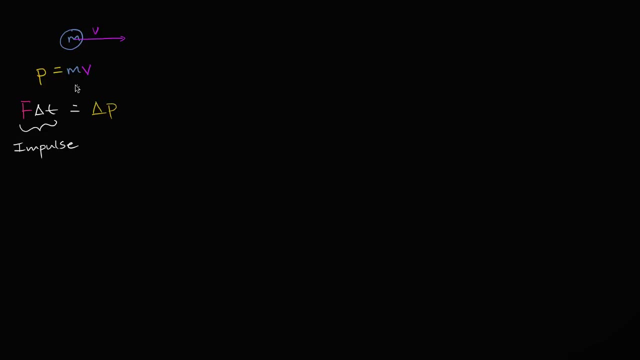 especially if you don't have any net force acting on an object, its momentum is going to be constant. You have a conservation of momentum And we use that idea in all sorts of interesting physics applications in the world, and especially in a lot of cases. 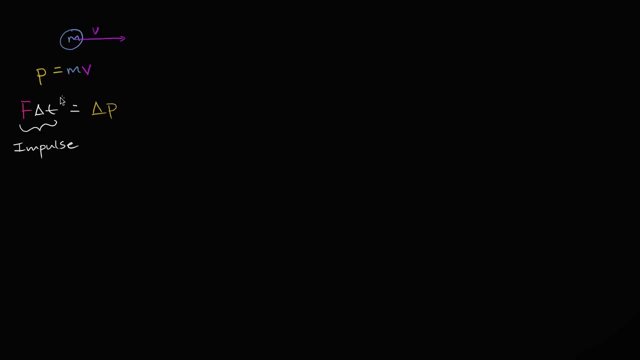 using billiard balls and whatever else. So now let's try to take a similar idea, but go into the rotational world. So let's imagine you have a mass And for the sake of this we're gonna assume it's a point mass. 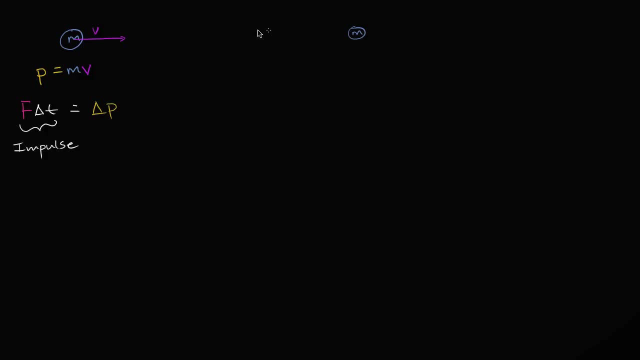 So you have a mass, a mass there, And let's just say it's attached by, essentially, a massless wire, a massless wire to it's just nailed down right over here, And so this right over here would be its center of rotation. 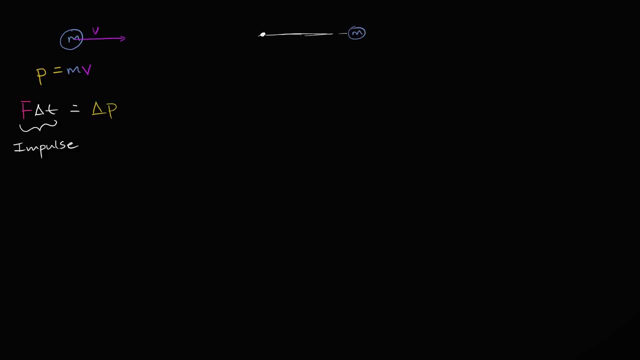 And so you could imagine if someone applied a torque to this mass. this mass could start rotating in a circle And you could just assume that it's maybe it's sitting on the screen. This is kind of a frictionless surface. There's no air resistance. 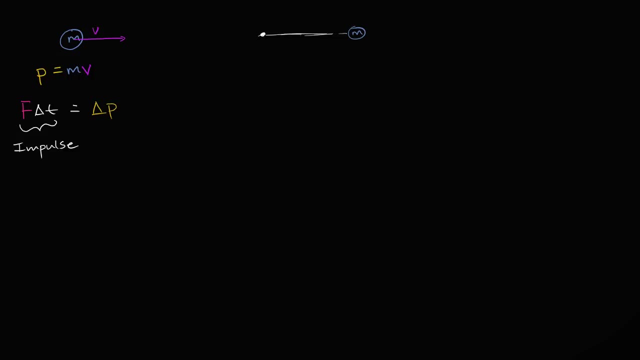 And so then it will if you apply a torque, if you apply a torque here, it will start rotating. And so you could think about: well, there might be an idea. just as momentum is this idea of well, how hard is it to stop something? 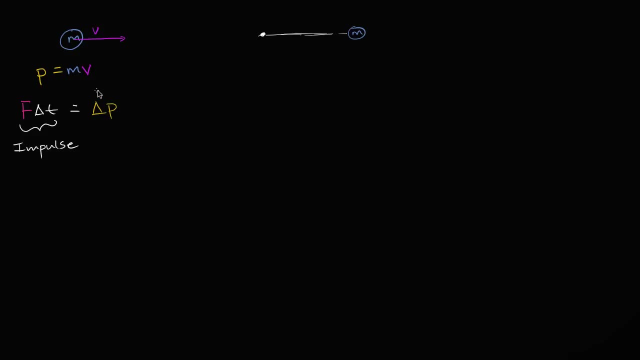 You might say: well, how- and this is stop translating something, something from moving. You might think, well, maybe there's a similar idea of how hard is it for something, or how hard is it to stop rotating something, And you could imagine that that idea has been defined. 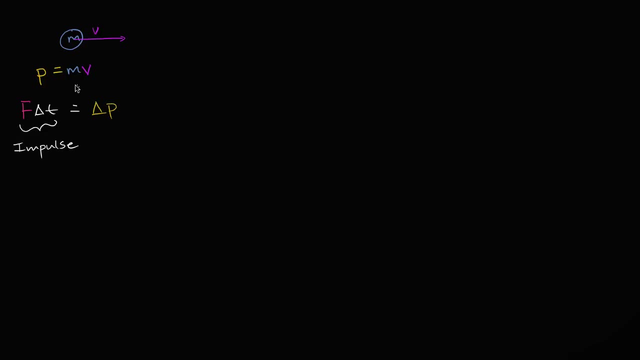 especially if you don't have any net force acting on an object, its momentum is going to be constant. You have a conservation of momentum And we use that idea in all sorts of interesting physics applications in the world, and especially a lot of cases using billiard balls. 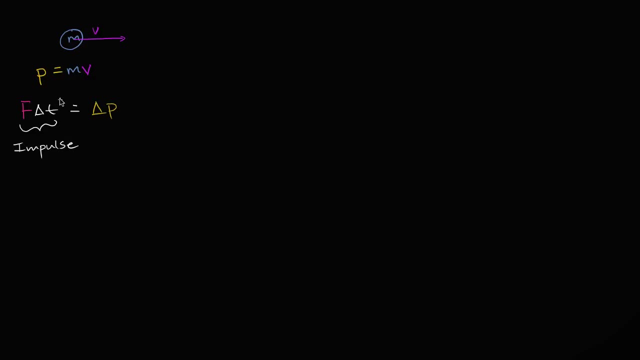 and whatever else. So now let's try to take a similar idea but go into the rotational world. So let's imagine you have a mass And for the sake of this we're gonna assume it's a point mass. So you have a mass. 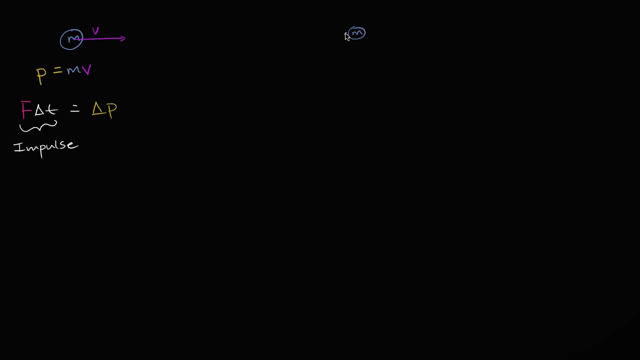 a mass there And let's just say it's attached by, essentially, a massless wire. a massless wire to it's just nailed down right over here, And so this right over here would be its center of rotation, And so you could imagine. 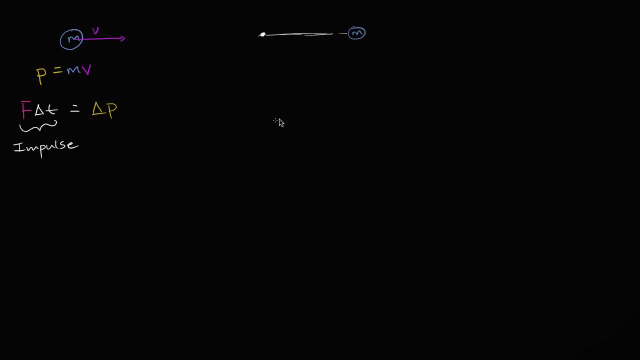 if someone applied a torque to this mass, this mass could start rotating in a circle And you could just assume that it's maybe it's sitting on the screen. This is kind of a frictionless surface. There's no air resistance, And so then it will. 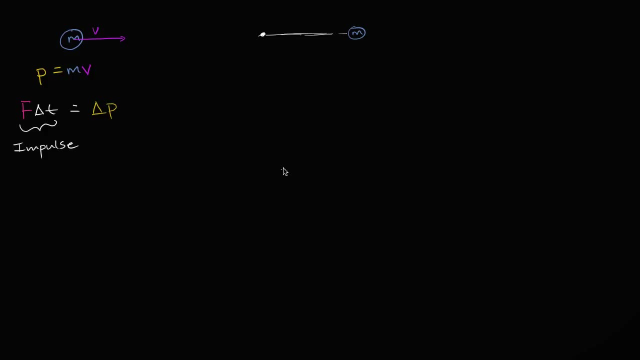 if you apply a torque, if you apply a torque here, it will start rotating. And so you could think about: well, there might be an idea. just as momentum is this idea of well, how hard is it to stop something? 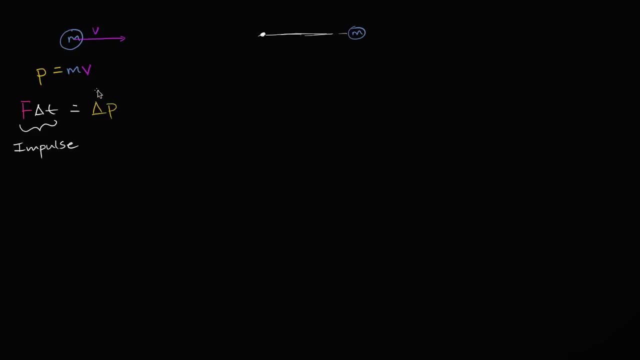 You might say: well, how- and this is stop translating something, something from moving. You might think, well, maybe there's a similar idea of how hard is it for something, or how hard is it to stop rotating something, And you could imagine that that idea has been defined. 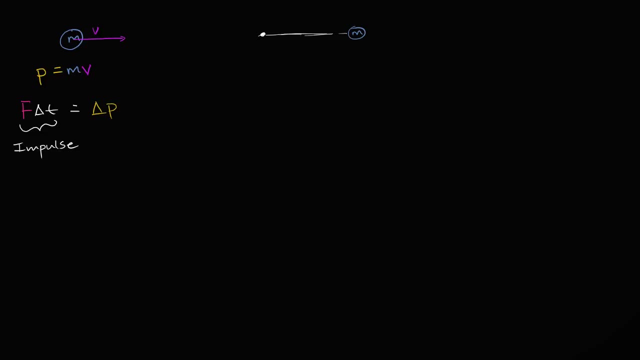 and it has been defined as angular momentum. So let me make this clear: This right over here is momentum, Mo momentum, And over here we'll talk about angular momentum, Angular angular momentum, Angular momentum, And actually both momentum and angular momentum. 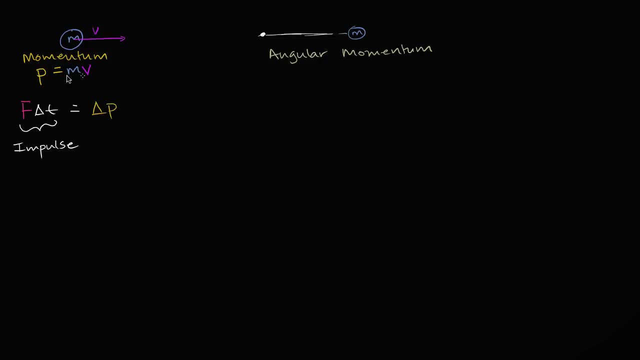 are vector quantities. So here I just wrote the kind of the magnitudes of velocity and momentum. But momentum is a vector and it could be defined. the momentum vector could be defined as equal to the mass, which is a scalar quantity. 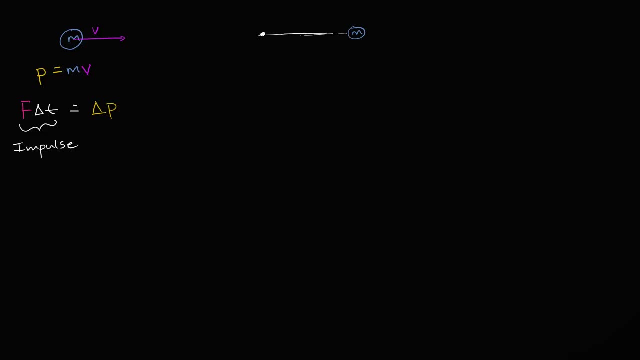 and it has been defined as angular momentum. So let me make this clear: This right over here is momentum, Mo momentum, And over here we'll talk about angular momentum, Angular angular momentum, Angular momentum, And actually both momentum and angular momentum. 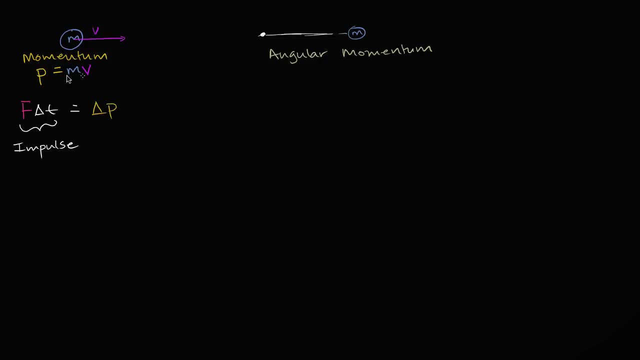 are vector quantities. So here I just wrote the kind of the magnitudes of velocity and momentum. But momentum is a vector and it could be defined. the momentum vector could be defined as equal to the mass, which is a scalar quantity. 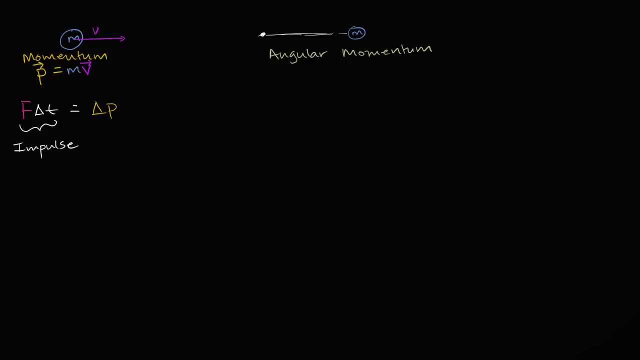 times the velocity, times the velocity vector. Now the same thing is true for angular momentum, but I'm gonna stay focused on the magnitude of angular momentum. Angular momentum can have direction, as you can imagine, You can rotate in two different ways. 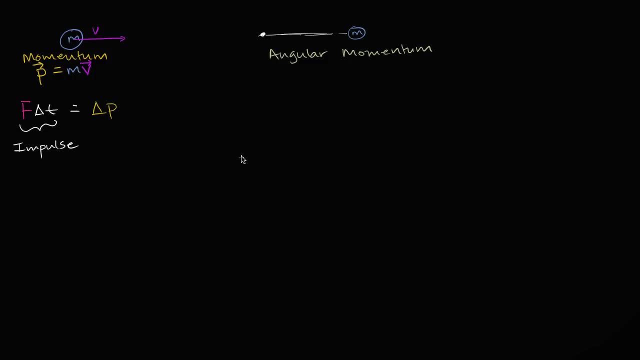 but that gets a little bit more complicated when you start thinking about taking the products of vectors because, as you may already know or you may see in the future, there's different ways of taking products of vectors. but just to get the intuition of angular momentum, 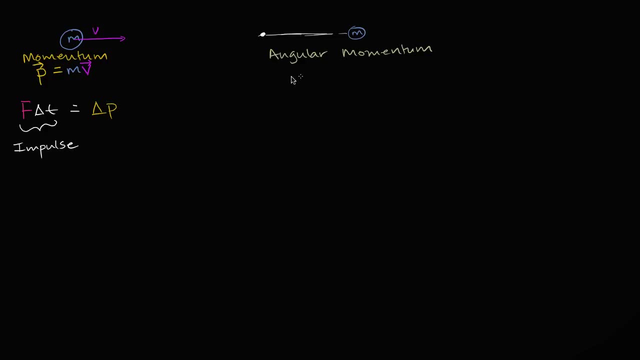 I'll focus on the magnitudes. So angular momentum is defined and the letter used is L. I did a lot of research to try to figure out why it is called L and I could not find a good reason, So in the message board below. 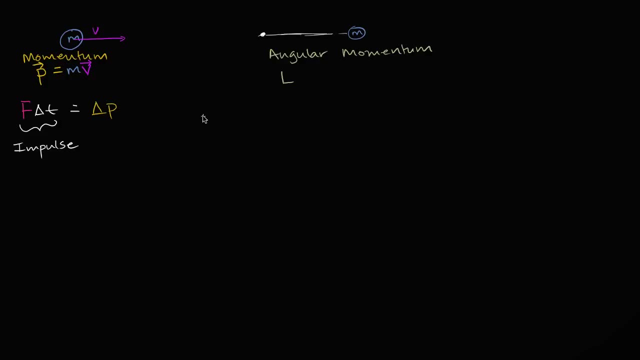 if anyone has a good reason, I would like to know why angular momentum is called L. A lot of the best arguments I saw is that almost everything else was all. the other letters were used up for other ideas. But anyway, angular momentum is defined. 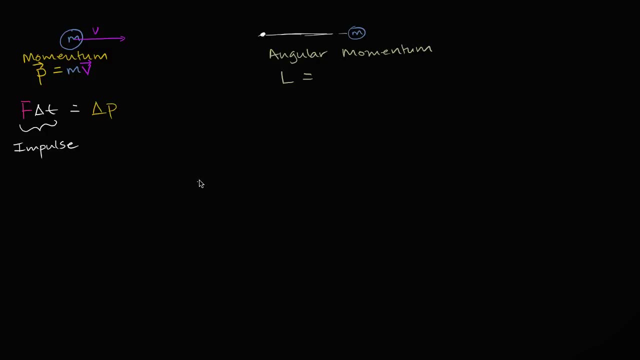 and it's defined very similarly. Just as kind of torque is a thing that can change how something rotates, and force is the way that something changes how something translates it, and torque is force times, distance from the center of rotation, everything in kind of the rotational world. 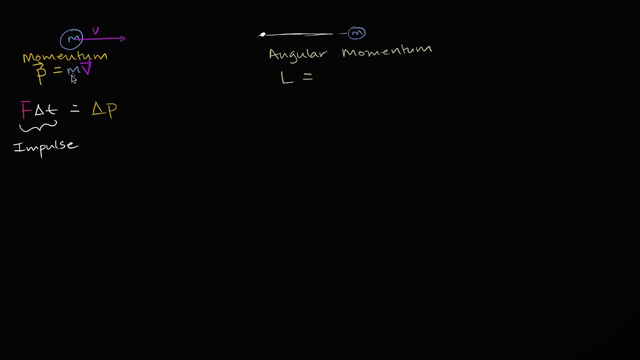 is defined in a similar way. You kind of take the analog and the translational world and you multiply: it times the distance from your center of rotation. So angular momentum is defined as. angular momentum is defined as mass times, velocity times, velocity times distance. 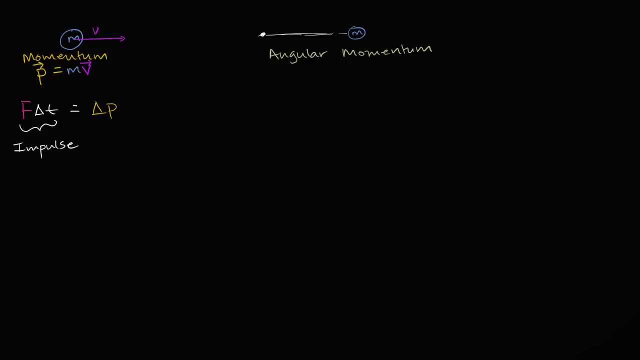 times the velocity, times the velocity vector. Now the same thing is true for angular momentum, but I'm gonna stay focused on the magnitude of angular momentum. Angular momentum can have direction, as you can imagine, You can rotate in two different ways. 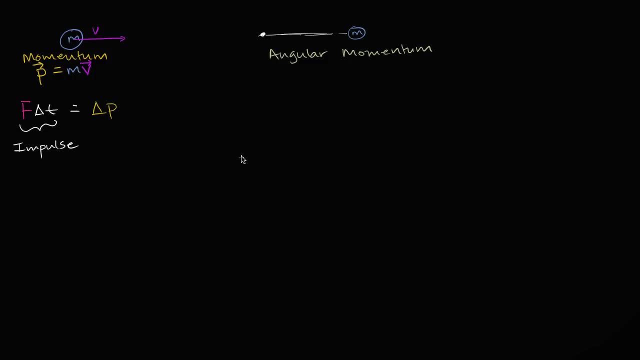 but that gets a little bit more complicated when you start thinking about taking the products of vectors because, as you may already know or you may see in the future, there's different ways of taking products of vectors. but just to get the intuition of angular momentum, 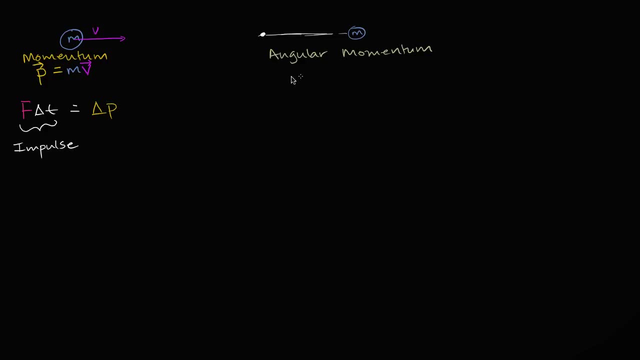 I'll focus on the magnitudes. So angular momentum is defined and the letter used is L. I did a lot of research to try to figure out why it is called L and I could not find a good reason, So in the message board below. 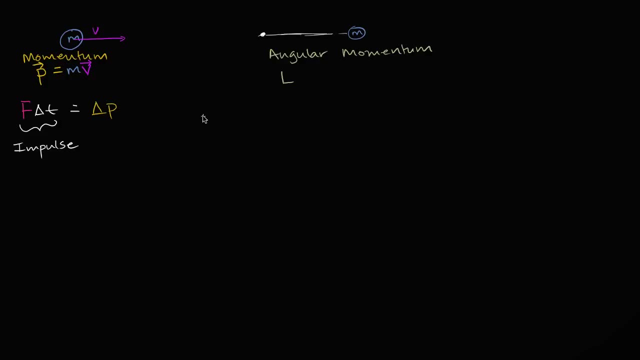 if anyone has a good reason, I would like to know why angular momentum is called L. A lot of the best arguments I saw is that almost everything else was all. the other letters were used up for other ideas. But anyway, angular momentum is defined. 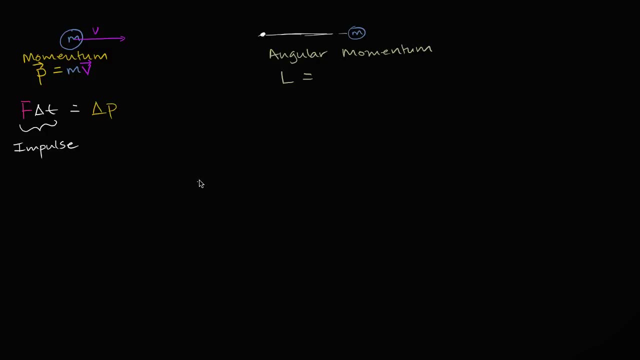 and it's defined very similarly. Just as kind of torque is a thing that can change how something rotates, and force is the way that something changes how something translates it, and torque is force times, distance from the center of rotation, everything in kind of the rotational world. 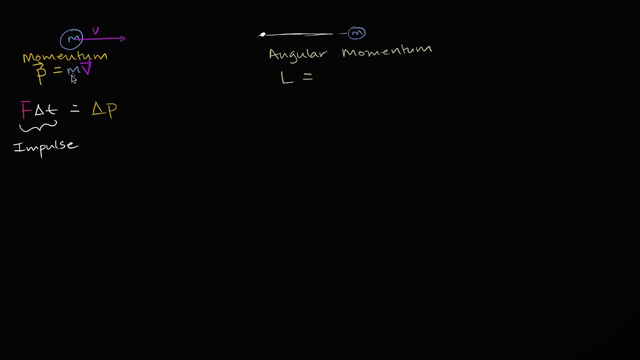 is defined in a similar way. You kind of take the analog and the translational world and you multiply: it times the distance from your center of rotation. So angular momentum is defined as. angular momentum is defined as mass times, velocity times, velocity times distance. 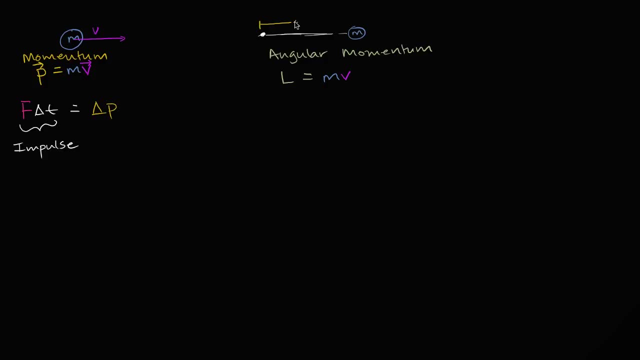 to from the center of rotation. So let's call this distance right over here r, R for radius, because you can imagine if this is traveling in a circle, that would be the radius of the circle mvr. Actually, let me be a little bit more careful here. 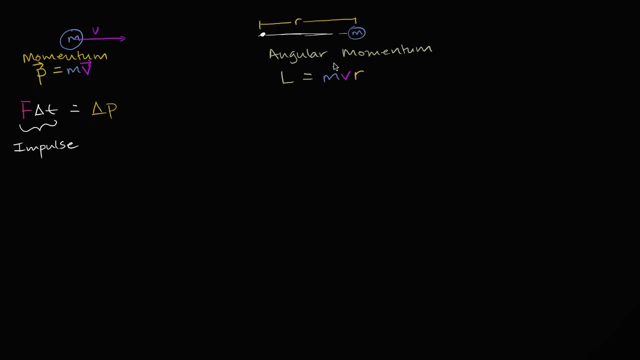 It's the magnitude of the velocity that is perpendicular to the radius. Sometimes it might be called the tangential velocity. So this symbol right over here, this is the magnitude of the velocity that is perpendicular to the radius. So it would be this: 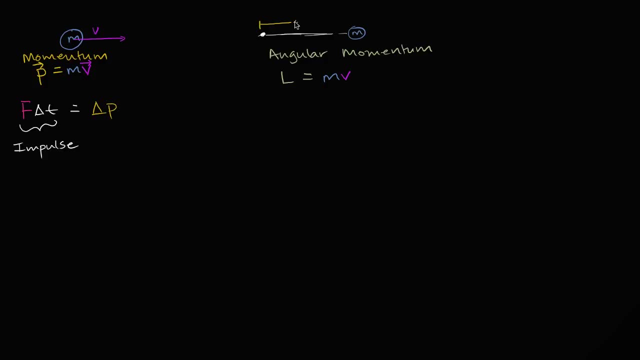 to from the center of rotation. So let's call this distance right over here r, R for radius, because you can imagine if this is traveling in a circle, that would be the radius of the circle mvr. Actually, let me be a little bit more careful here. 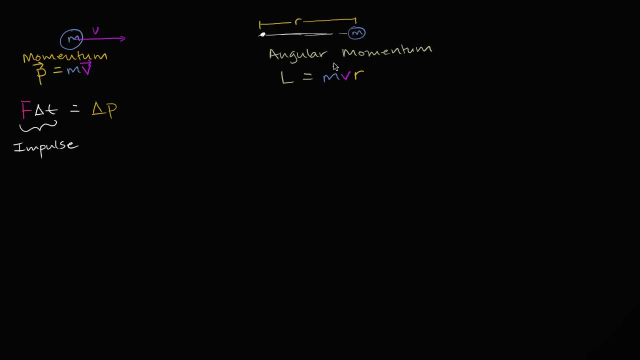 It's the magnitude of the velocity that is perpendicular to the radius. Sometimes it might be called the tangential velocity. So this symbol right over here, this is the magnitude of the velocity that is perpendicular to the radius. So it would be this: 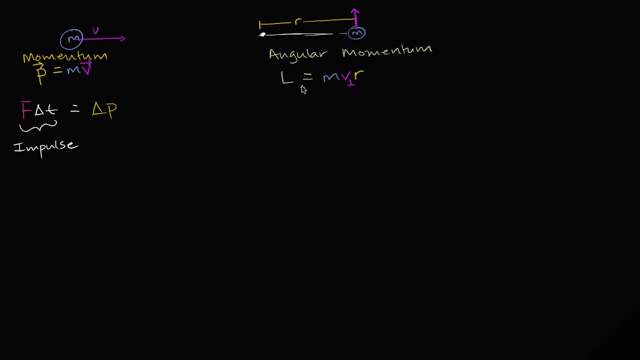 it would be that magnitude right over here. This is what we define as angular momentum, And what I will tell you here is, just as, in the absence of a net force, momentum is constant. we know and we know that momentum is constant. 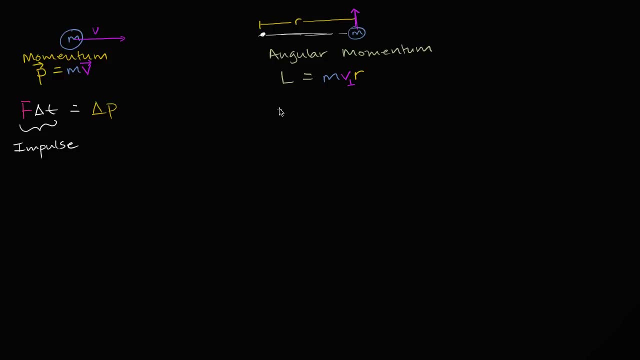 we know, and we know that momentum is constant. we know, and I haven't shown it to you yet, I haven't proven it to you yet mathematically, but in the absence of torque. so if torque is equal to zero, 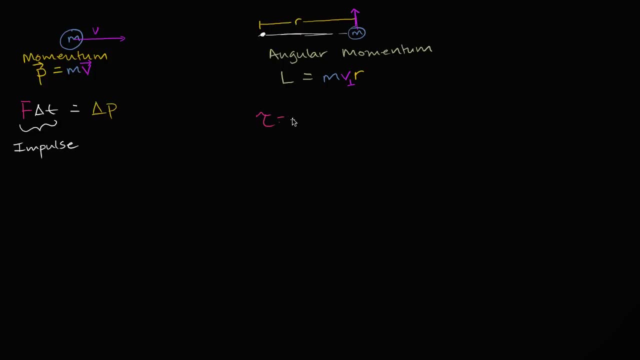 we do torque in pink. if torque is equal to zero, if there's no net torque going on here, if the magnitude of torque is equal to zero, then we will have, then we will have no change, no change in angular momentum. 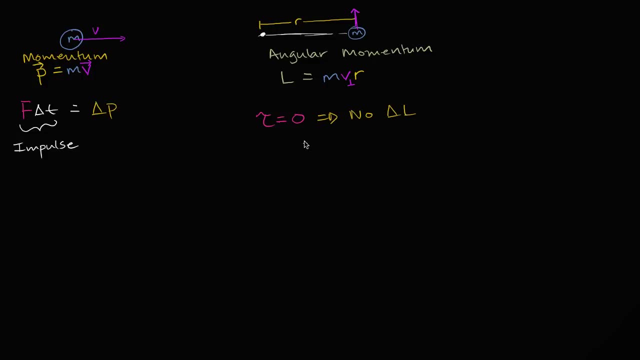 And we will look at that mathematically in a few seconds, But just from this there's a very interesting thing that arises, and something that you might have observed at even the Olympics or in other things, And this is the idea that you can. 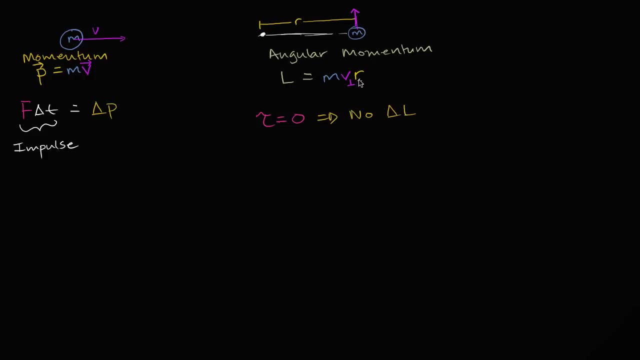 by changing your radius, you could actually change your tangential velocity And, as we've seen in previous videos, tangential velocity is closely related to angular, to angular velocity. So let's explore that a little bit. So when we write it, 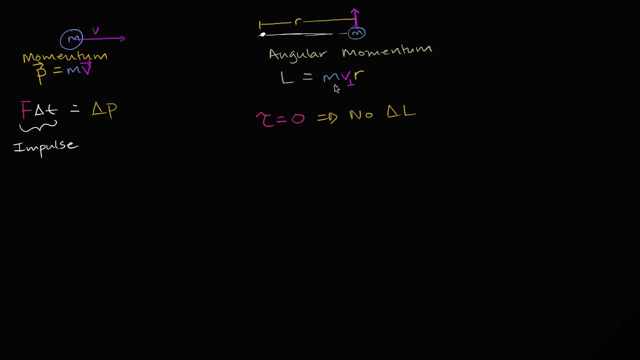 in the world where, well, actually, you see it straight out of this: if L is constant, if R went down, so let me write this down, So let me rewrite it over here. So L whoops, So let me write it. 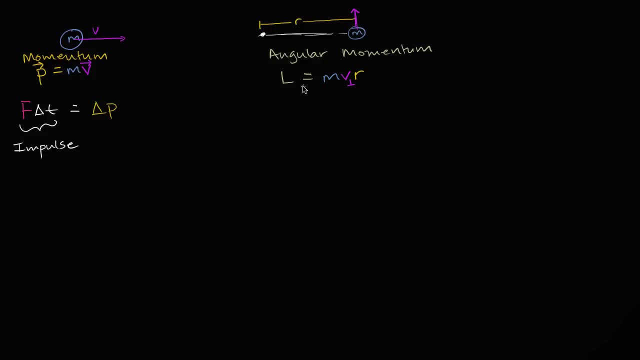 it would be that magnitude right over here. This is what we define as angular momentum, And what I will tell you here is, just as, in the absence of a net force, momentum is constant. we know and we know that momentum is constant. 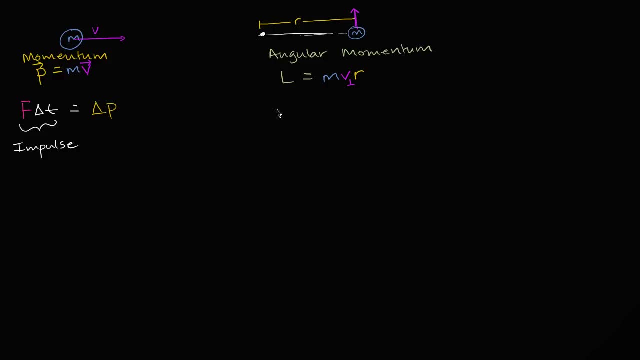 we know, and I haven't shown it to you yet, I haven't proven it to you yet mathematically, but in the absence of torque. so if torque is equal to zero, we do torque in pink if torque is equal to zero. 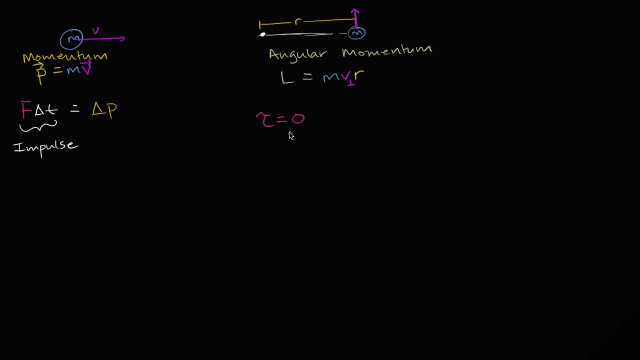 if there's no net torque going on here, if the magnitude of torque is equal to zero, then then we will have, then we will have no change, no, no change in angular momentum, And we will look at that mathematically. 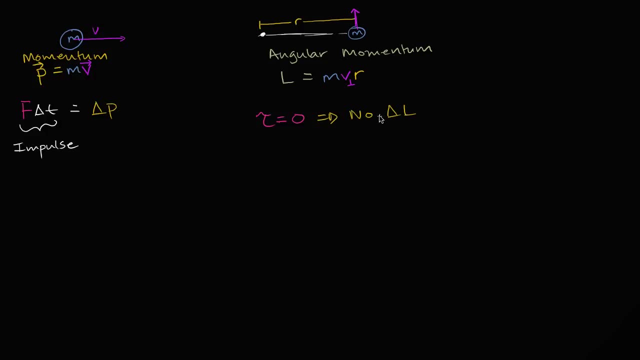 in a few seconds. But just from this, there's a very interesting thing that arises, and something that you might have observed at even the Olympics or in other things, And this is the idea that you can- by changing your radius, you could actually change your tangential velocity. 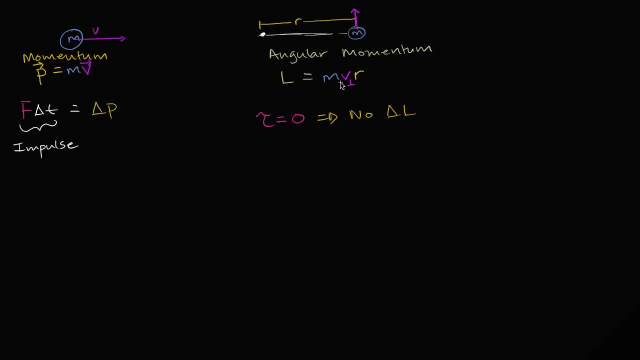 And, as we've seen in previous videos, tangential velocity is closely related to angular, to angular velocity. So let's explore that a little bit. So when we write it in the world, where well, actually, you see it straight out of this. 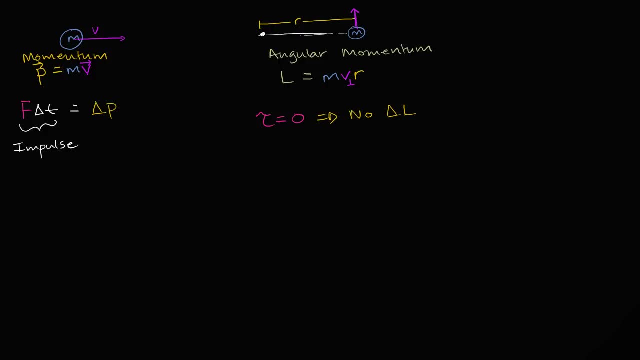 if L is constant, if R went down, so let me write this down, so let me rewrite it over here. So L, whoops, so let me write it. L is equal to mass times, tangential velocity, or actually, well, yeah, tangential velocity. 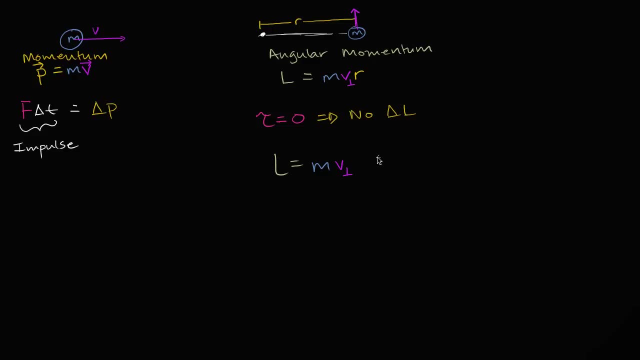 or the velocity that's perpendicular to the radius times, the radius. Now, what happens if we assume that this is constant, If we assume that this is- let me write this down- If we assume that there's no torque, so we're in this world. 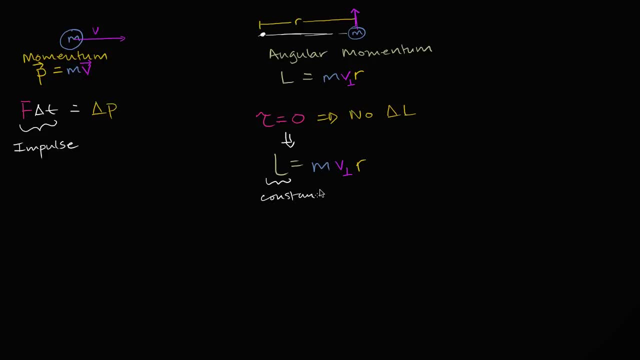 so this over here is going to be constant. This is going to be constant. So what happens if we were to reduce R, if somehow, you know, this wire started to reel in a little bit or started to wrap around here, and actually that's actually a reasonable thing? 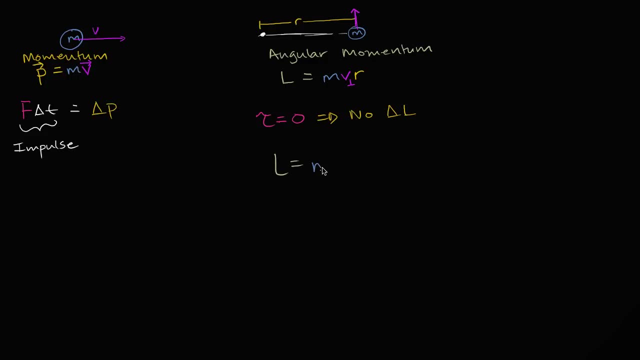 L is equal to mass times, tangential velocity, or actually, well, yeah, tangential velocity, or the velocity that's perpendicular to the radius times. the radius, Now, what happens if we assume that this is constant, If we assume that this is? 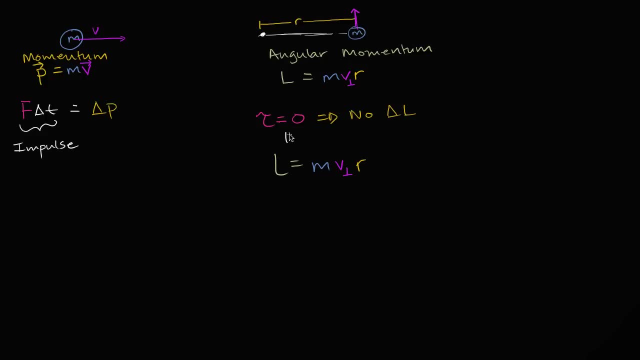 let me write this down. If we assume that there's no torque, so we're in this world, so this over here is going to be constant. If this is going to be constant, So what happens if we were to reduce R, If somehow this wire started to reel in a little bit? 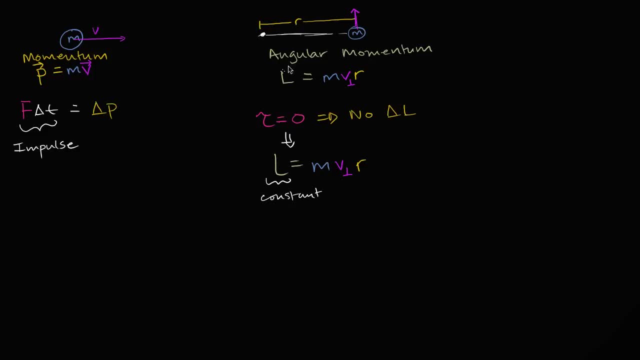 or started to wrap around here, And actually that's actually a reasonable thing, You can imagine. as it rotates, it starts to wrap around this thing, so the wire gets shorter. So if R goes down, if R goes down, and this is constant, 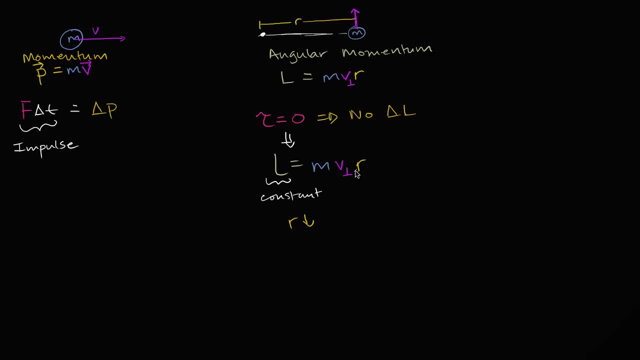 the mass isn't going to change. Well, if L is constant, mass isn't changing. R is going down. tangential velocity, or the velocity that's perpendicular to the radius, is going to go up Velocity that is perpendicular to the radius. 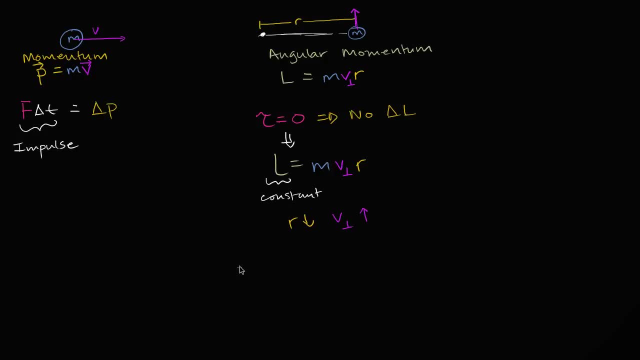 is going to go up And if we want to think about it- and we can think about it in terms of angular velocity, we know that angular velocity, which we would measure in radians per second, we would use the symbol omega. omega is defined. 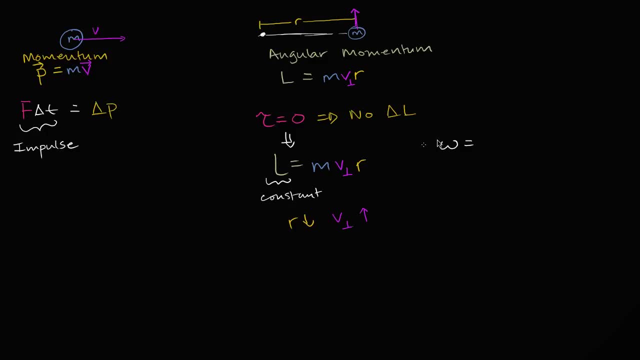 and we go into much more depth in this in other videos- as tangential velocity. tangential velocity, the magnitude of the velocity that is perpendicular to the radius divided by the radius. Divided by the radius, Or, if you solve for tangential velocity, 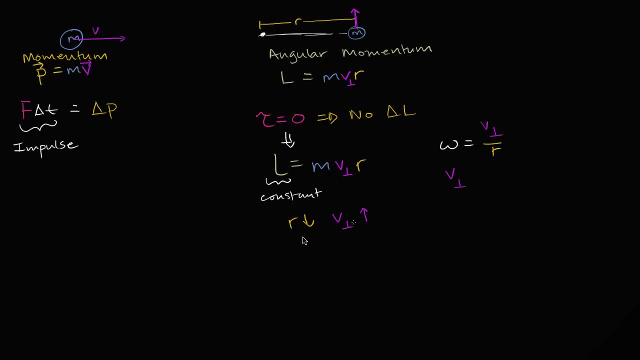 you get: V is equal to, is equal to omega R Is equal to omega omega R. And so if you substitute back into this, really this definition for angular momentum, you get angular momentum is equal to mass times, this times R, So mass times. 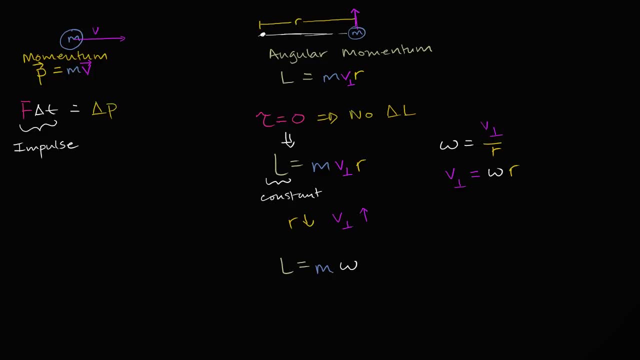 I'm just substituting for velocity here: times omega R, omega R, times R, Which of course is just omega omega R squared. So once again we do the same exercise. If our radius goes down, what happens to our angular velocity? 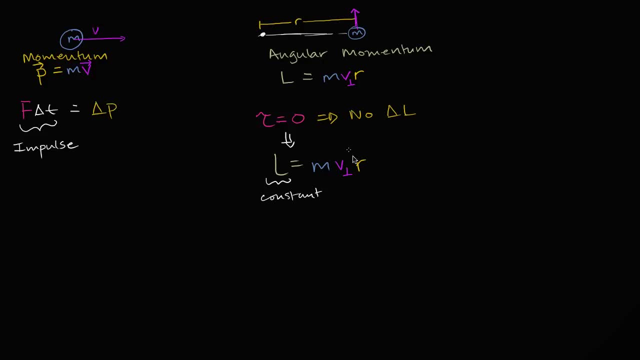 You can imagine, as it rotates, it starts to wrap around this thing, so the wire gets shorter. If r goes down, and this is constant, the mass isn't going to change. Well, if l is constant, mass isn't changing. 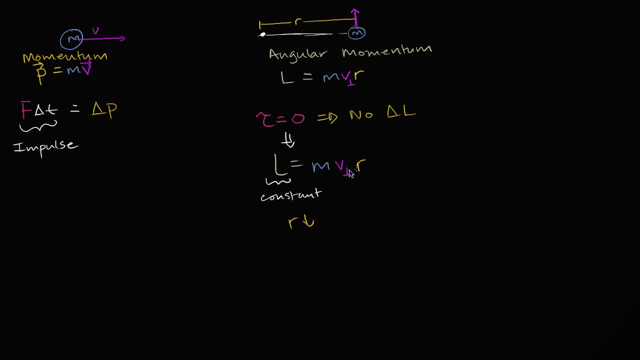 r is going down. tangential velocity, or the velocity that's perpendicular to the radius, is going to go up. Velocity that is perpendicular to the radius is going to go up And if we want to think about it, and we can think about it in terms of angular velocity, 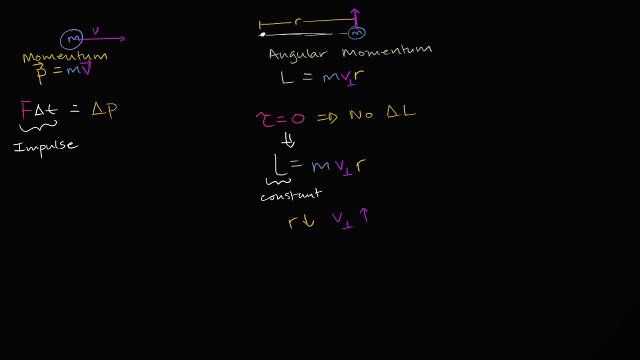 we know that angular velocity, which we would measure in radians per second, we would use the symbol omega. Omega is defined- and we go into much more depth in this in other videos- as tangential velocity. tangential velocity: the magnitude of the velocity. 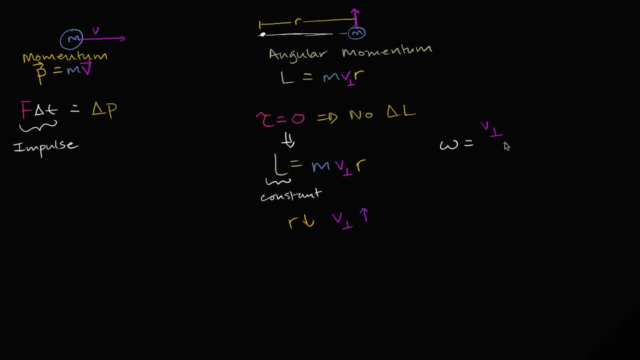 that is perpendicular to the radius divided by the radius, Divided by the radius. Or, if you solve for tangential velocity, you get: v is equal to, is equal to omega r, Is equal to omega, omega, omega r. And so if you substitute back into this, 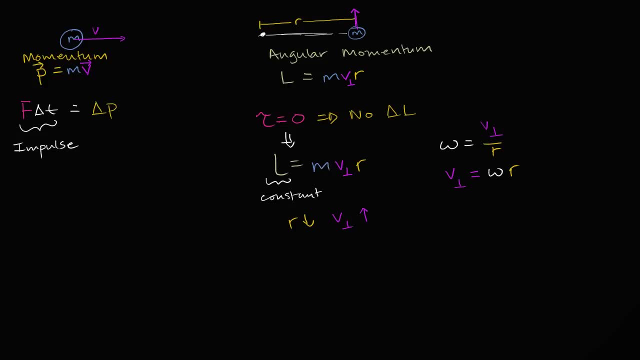 really this definition for angular momentum you get. you get: angular momentum is equal to mass times. this times r, So mass times. I'm just substituting for velocity here: times omega r, omega r, times r, Which of course is just omega- omega r squared. 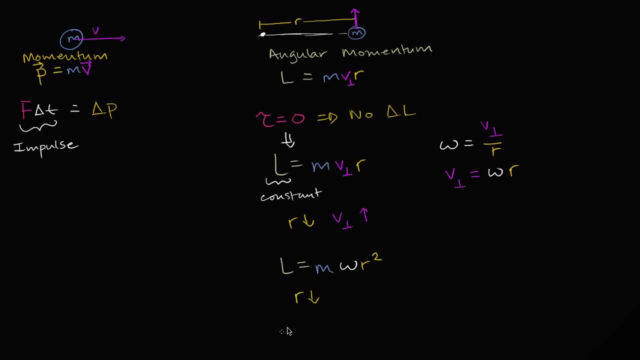 So, once again, we do the same exercise. If our radius goes down, what happens to our angular velocity? Remember, we could measure this in angles per second or radians per second. Well, if this goes, if this is constant- remember, we're assuming that there's no net torque- 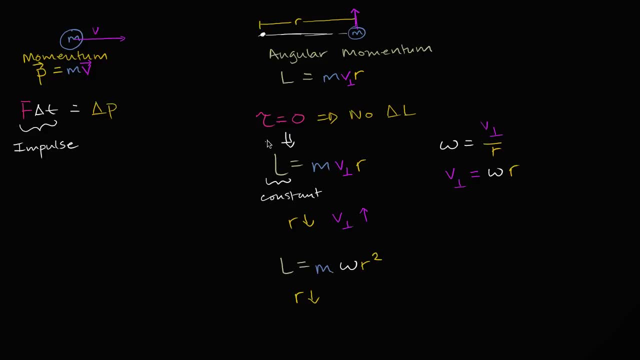 being applied to the system. so we're still in. we're still in this world right over here. If we assume that this thing is it's changing, but the radius were to change, what's going to happen to omega? Well, omega is going to go. 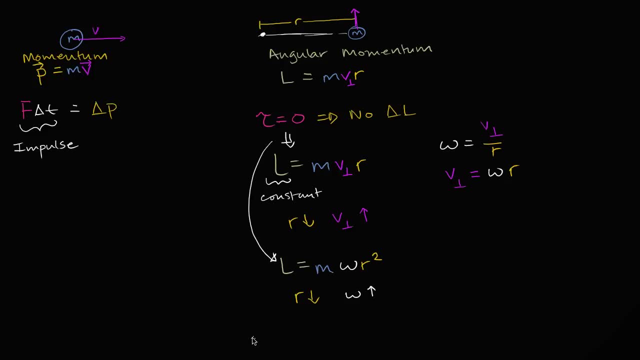 omega is going to go up Now. likewise, if the radius got longer- if the radius got longer, so the radius got longer- what's going to happen to omega? Omega is going to go. omega is going to go down. So if you reduce the radius,